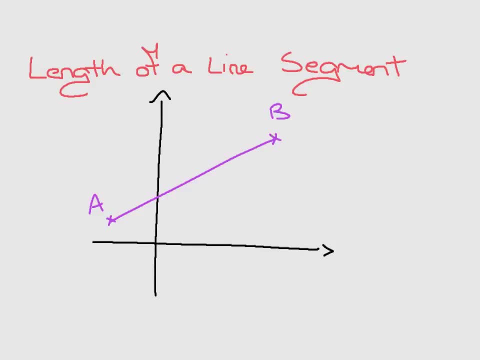 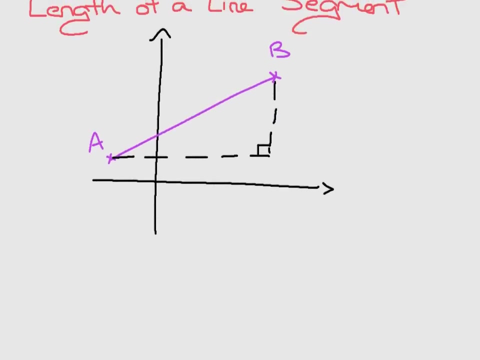 The thing to realize here is that if we look at the horizontal distance between points A and B, which I'm drawing right now, as well as the vertical distance between A and B, what we've just made here is a right angle triangle. So if I now, on this same graph, were to label the sides, and let's say, I call this side length C, I'll call this side length A. 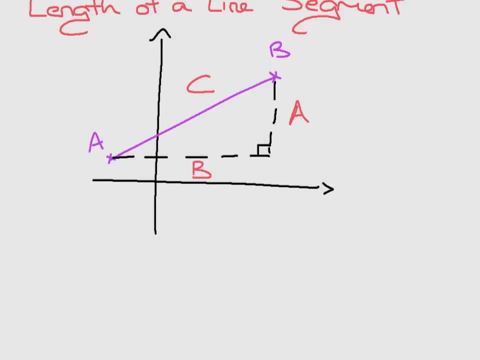 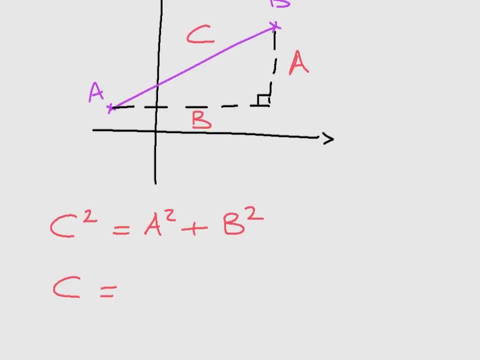 and I'll say: let's call this one B. then Pythagoras's theorem, which we all know, tells us that C squared is equal to A squared plus B squared. This then leads us to the fact that C will be equal to the square root of A squared plus B squared. 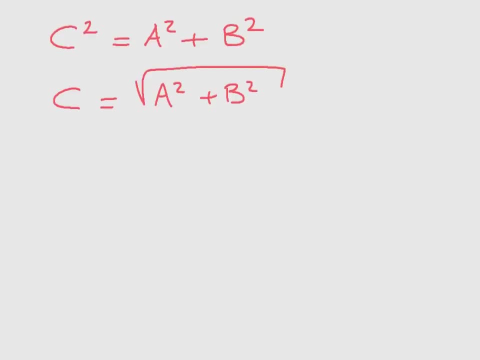 That's Pythagoras's theorem. Now, if I draw another one of these diagrams- Pythagoras still the quick x-y grid here, and I'll draw another segment with two endpoints and I'll call that A and B again. 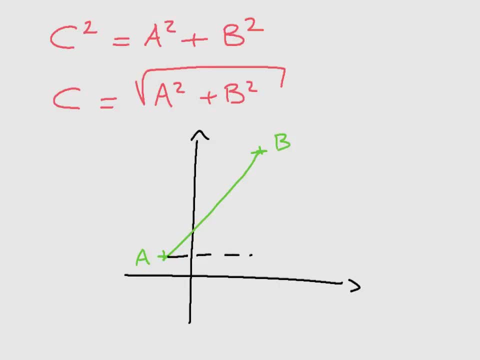 The trick is to realize that this distance here, the horizontal step and the vertical step here, are both given by two quite simple formulas. If I look at the coordinates of A and the coordinates of B, what we'll do here is that we'll say that A has coordinates x1, y1,. 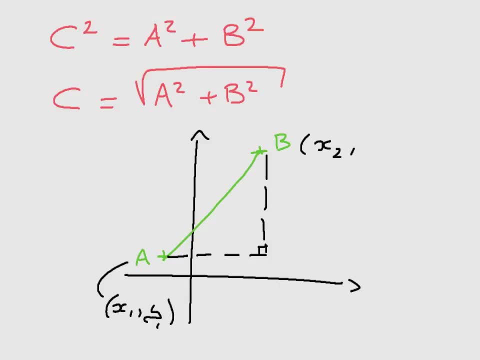 and B has coordinates x2, y2. Then the vertical step, which I'm pointing towards right now, is going to be equal to the difference in the two y-coordinates. In other words, that's y2 minus y1. And the horizontal step will be equal to the difference between the two x-coordinates. 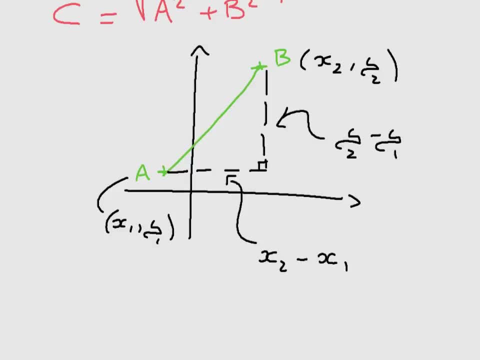 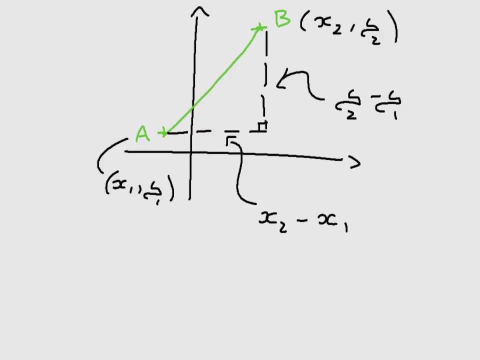 which will be equal to x2 minus x1.. And so, using what we saw before with Pythagoras's theorem, we can now rewrite our formula in the following way: If I write the length of the line, segment AB, squared, that would be equal to the horizontal step.